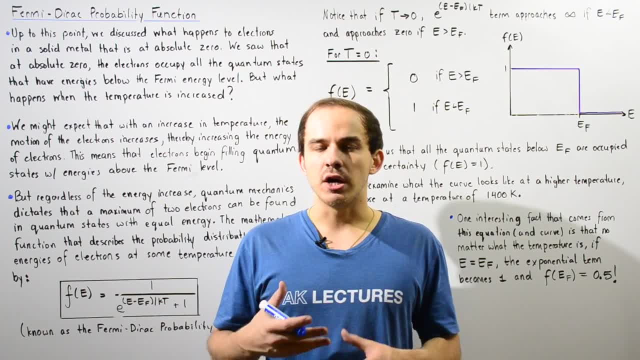 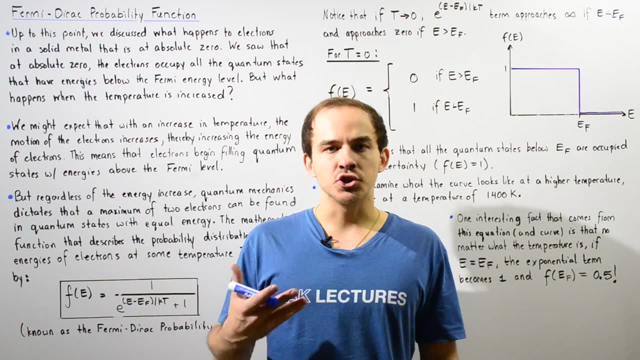 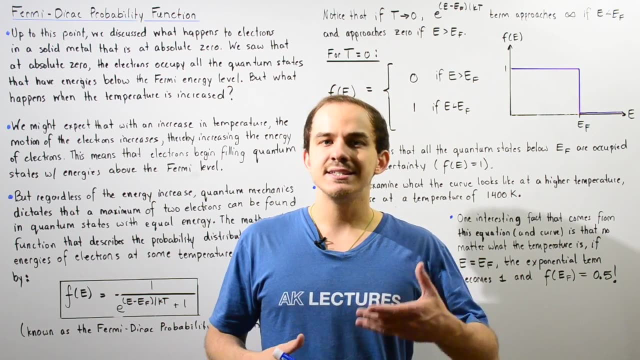 Up to this point in our discussion on electrons found inside solid metals. we examined what happens to our electrons when the temperature is at absolute zero, when the temperature of the metal is at absolute zero, that is, zero kelvins. So we basically saw that if the temperature is at zero, 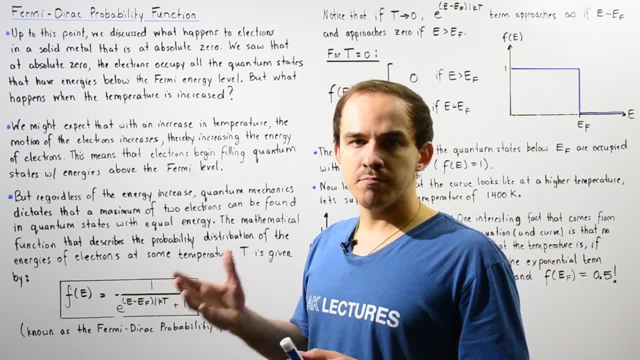 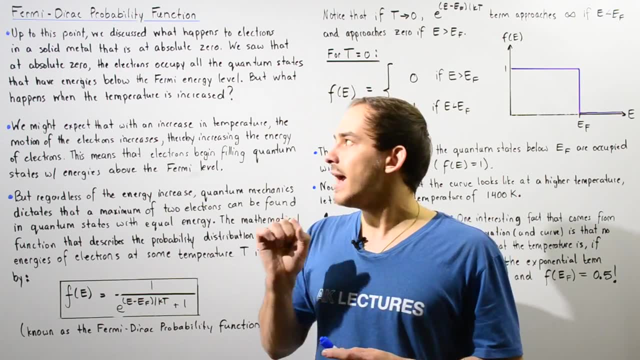 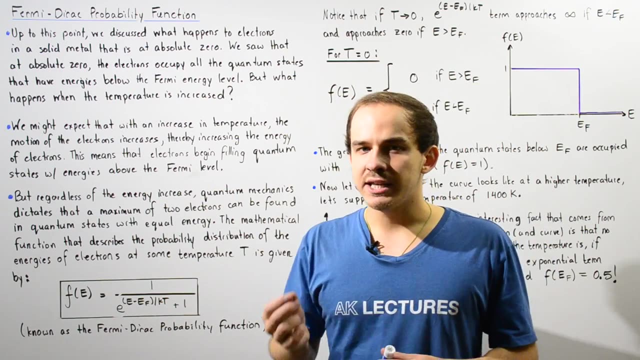 kelvins. the electrons inside our solid metal will occupy all the possible quantum states that have energies below the energy given by the Fermi energy level. Now the question still remains what exactly happens to our electrons when we increase the temperature to a temperature above? 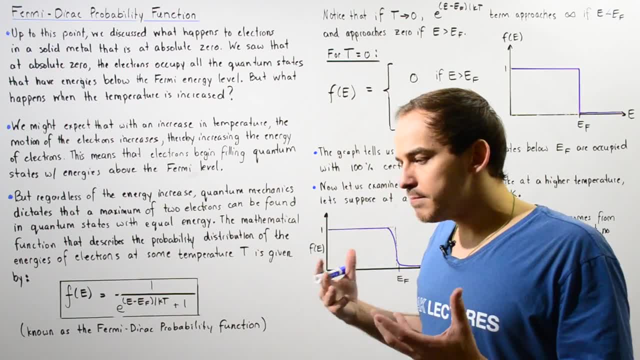 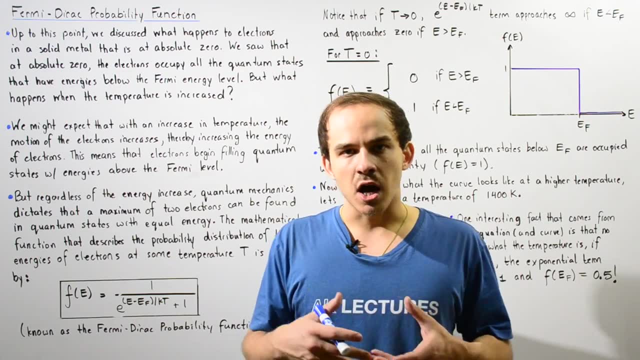 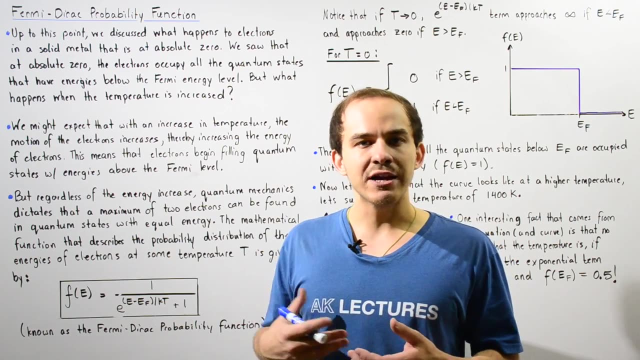 absolute zero. So we might make a prediction. So basically, when we increase the temperature to a temperature above absolute zero, that means our electrons on average will move more vigorously. So we're going to increase the general motion of our electrons by increasing our temperature. Now that means we basically 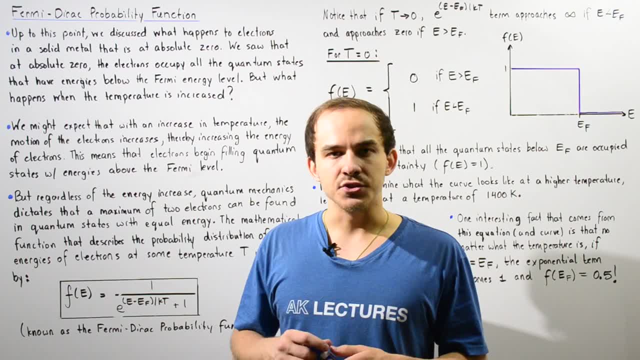 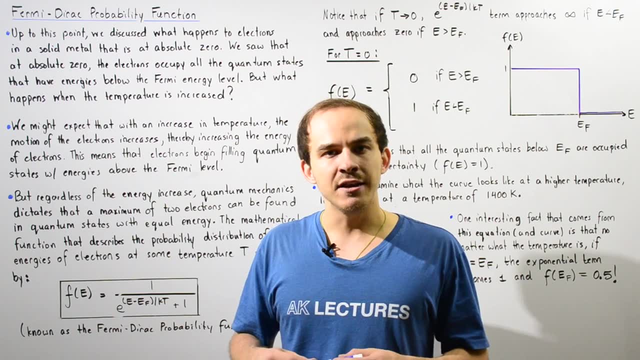 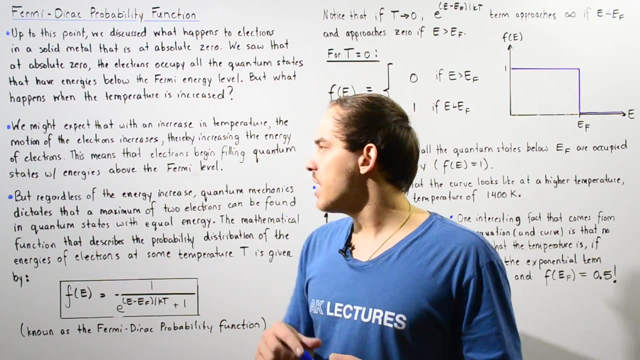 increase the thermal energy of our electrons, And so that might mean that as we increase the temperature, the electrons might have enough energy to actually jump to energy quantum states That have energies greater than the Fermi energy level. So once again, we might expect that with 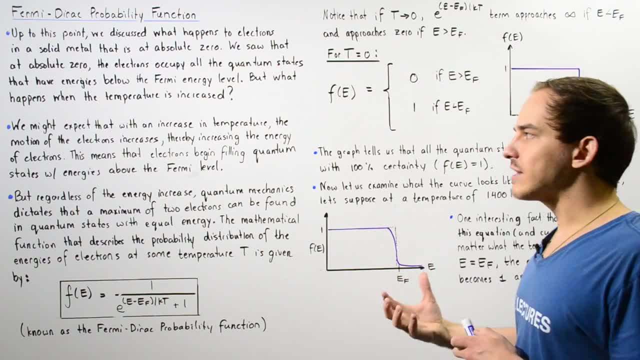 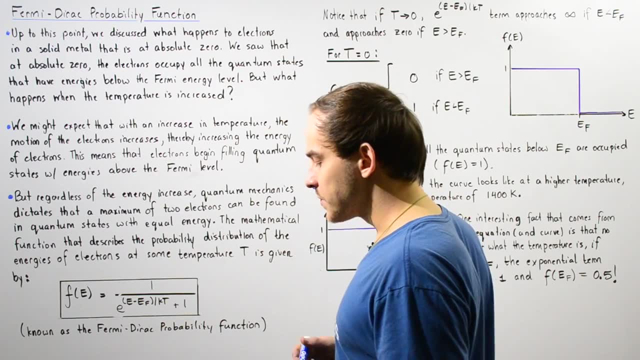 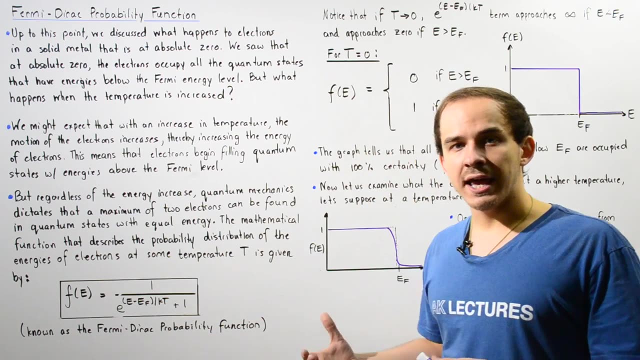 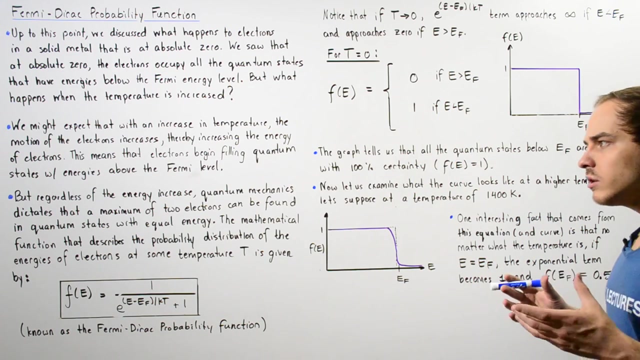 an increase in temperature, the motion of our electrons increases, thereby increasing the energy of our electrons, the thermal energy of our electrons, And this means that the electrons begin filling the quantum states that have energies which are above the Fermi energy level. Now, regardless of how our electrons' energy changes or increases, quantum mechanics and 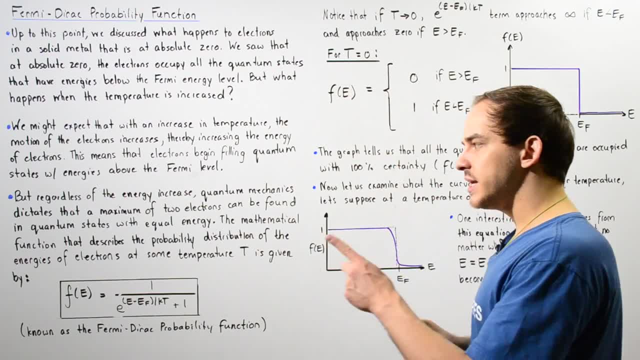 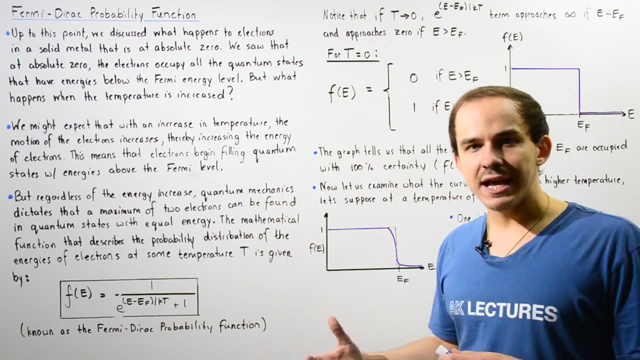 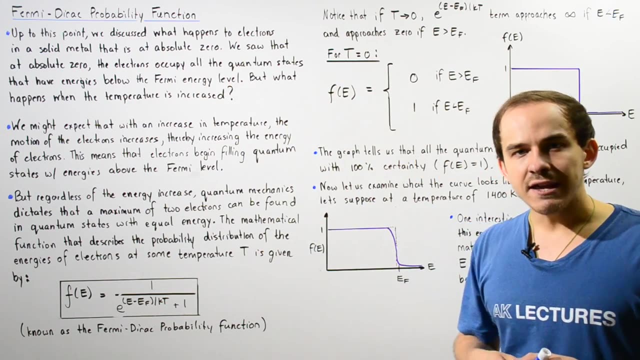 specifically, the Pauli exclusion principle dictates that a maximum of two electrons can be found in any quantum state that has the same equal energy. So basically, Pauli exclusion principle tells us that if the first three quantum states have the same equal energy, then the maximum of two electrons 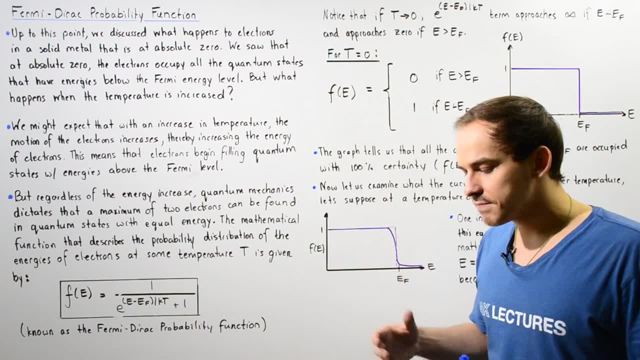 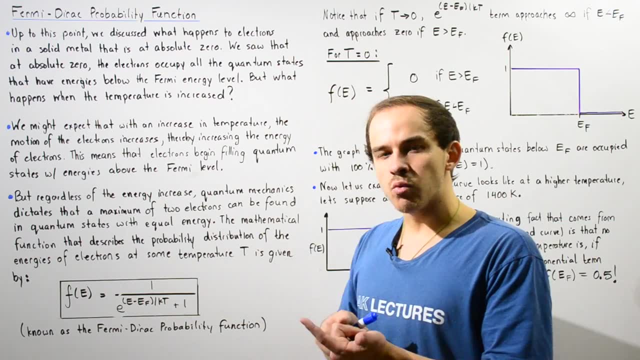 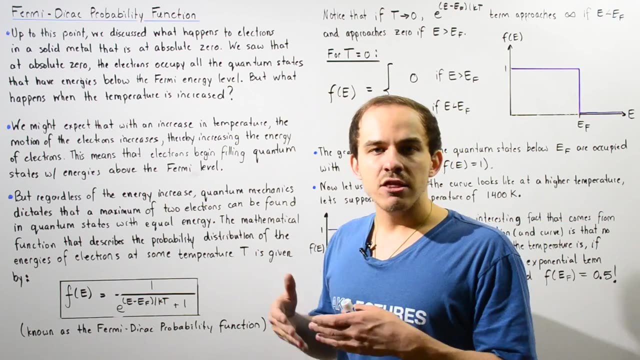 can be found within that quantum state. So if we have the same exact principal quantum number, orbital quantum number and magnetic quantum number, a maximum of two electrons can be found within that quantum state, And those electrons, electron spin, will be opposite. So one electron. 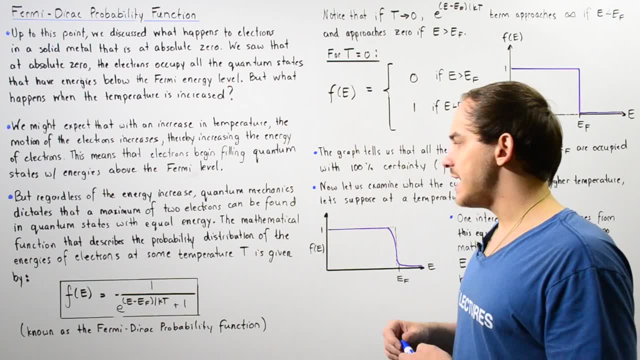 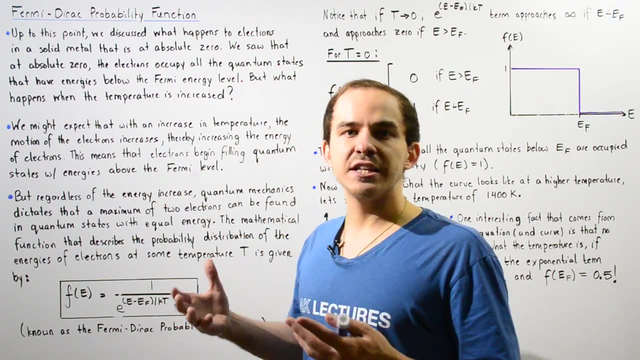 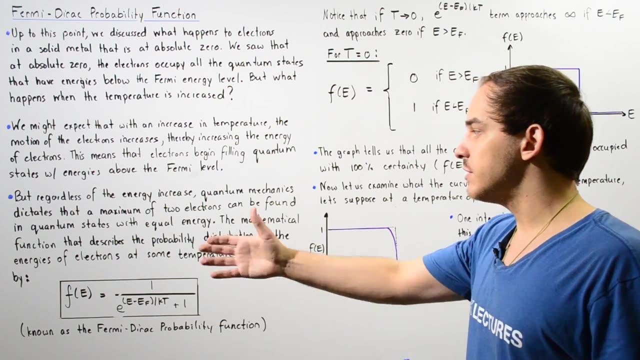 will have a positive one-half. the other electron will have a negative one-half. electron spin, The mathematical function, the equation that basically describes the probability distribution of the energies, of the quantum state energies of the electrons at some temperature, T, is given by the following equation: 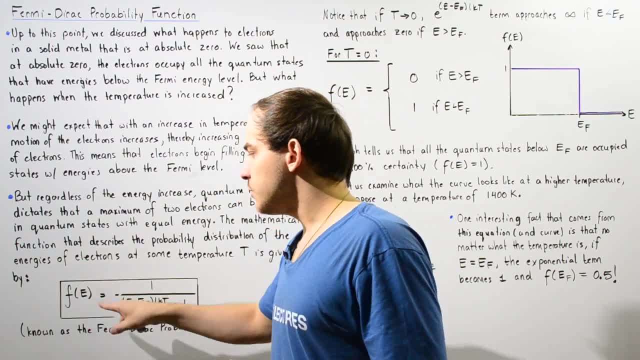 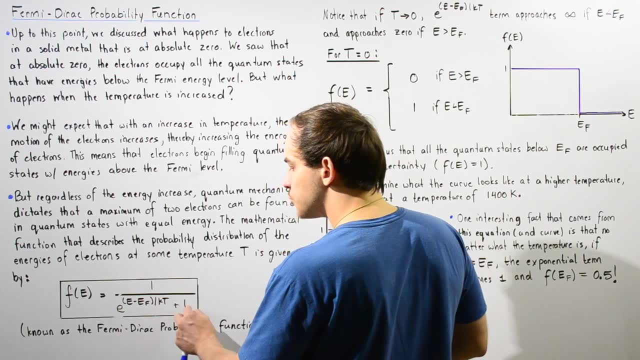 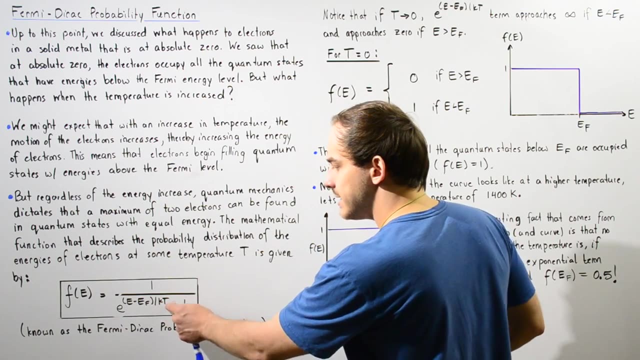 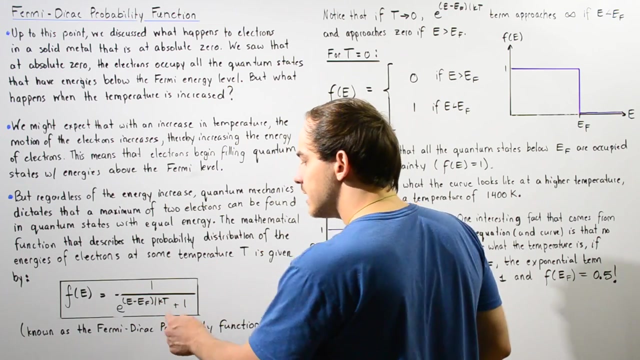 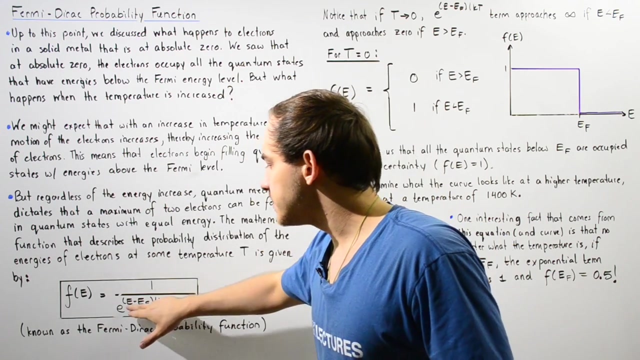 So F of E, where the probability distribution depends on the energy E of our electron, is equal to 1 divided by this term plus 1.. So we have our E to the power of E minus EF, divided by KT, where this lowercase E is simply our exponential function. this K is the Boltzmann constant, this T is the temperature in kelvins, this EF is our Fermi energy level and this E is simply our energy of our electron. 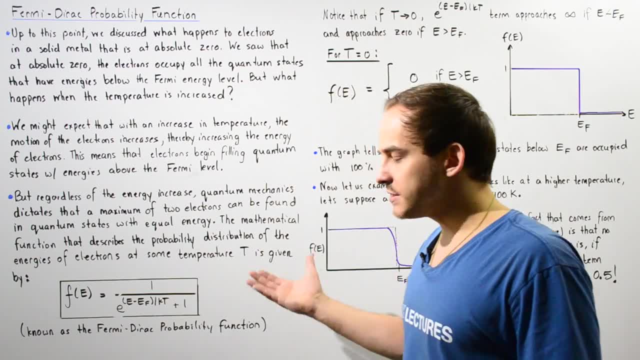 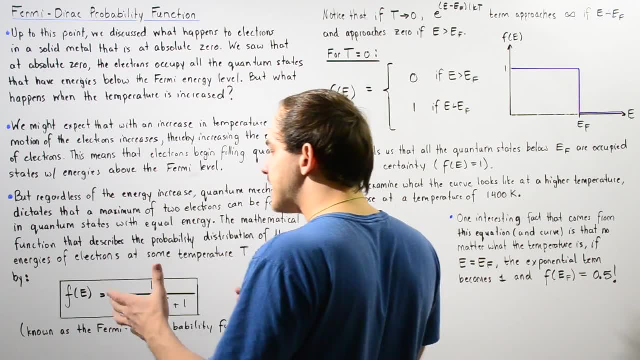 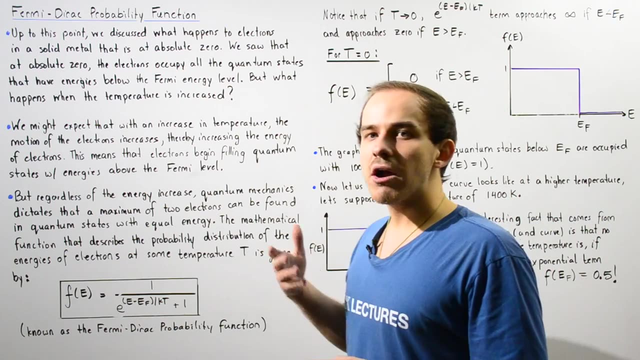 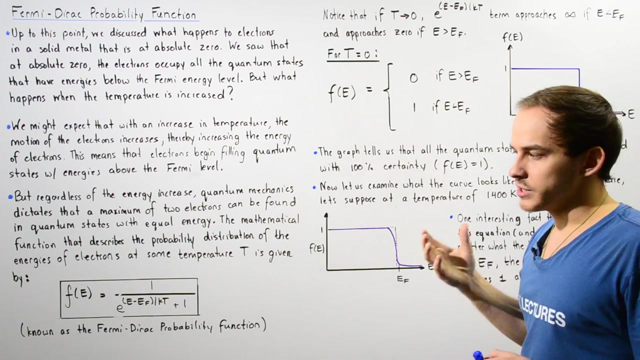 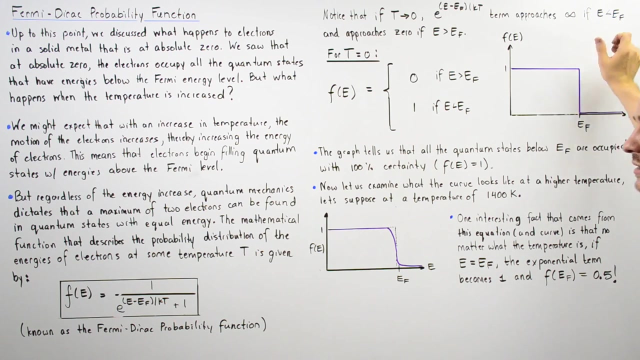 Now this equation has a name, and this is commonly known as the Fermi. So let's begin by taking this equation and asking ourselves: what exactly does this equation actually tell us when our temperature is very close to zero? So, basically, we see that as our temperature T approaches absolute zero, if our E value is less than the Fermi level, we see that this exponent of the exponential 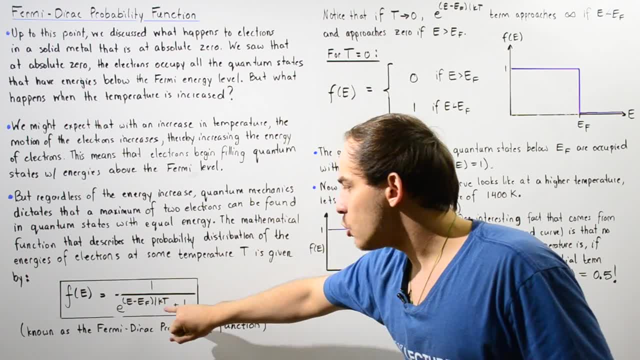 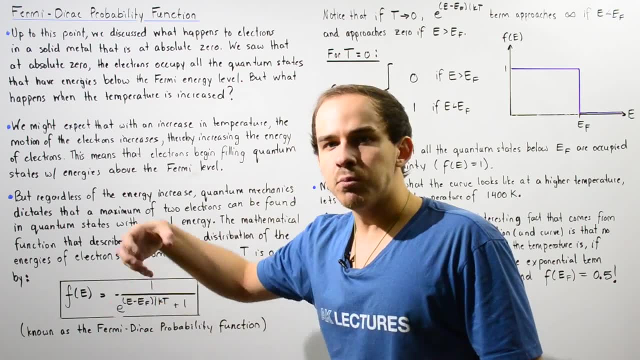 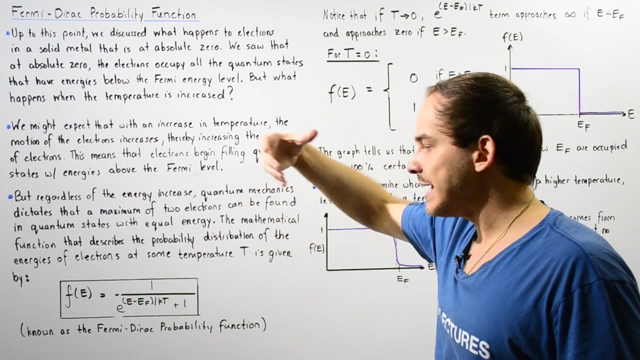 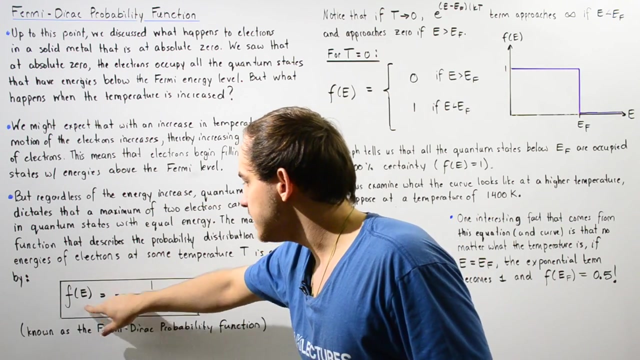 function becomes negative. and so if this K term is very, very small, that means this exponential term approaches infinity. And so if the exponential term approaches infinity, 1 divided by an infinitely large number is very close to zero. So for such a case, we see that F of E is simply equal to 1 divided by zero plus 1, or simply 1 divided by 1.. 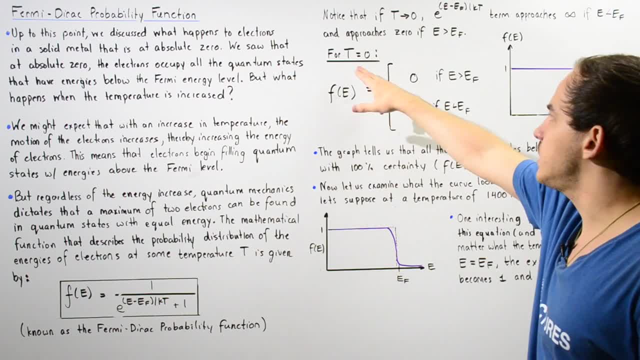 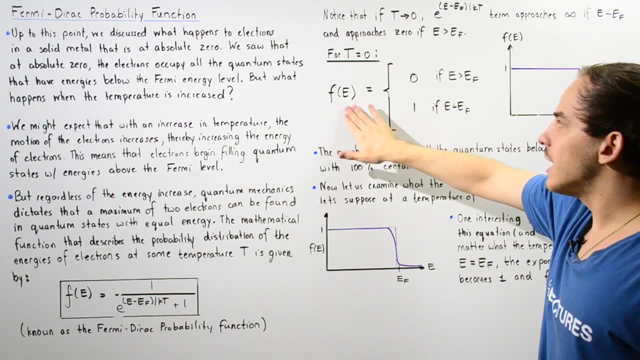 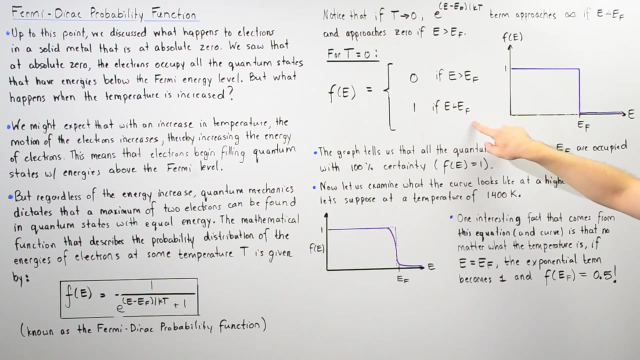 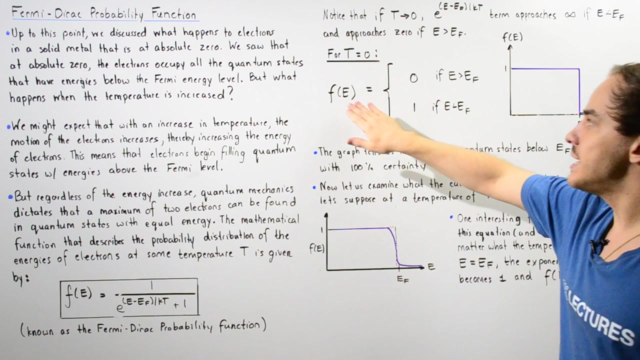 Which is equal to 1.. So we see, for a temperature that is very close or equal to zero, we see or we define the following probability distribution. So if our E is less than EF, if the Fermi level is greater than our energy E of that electron, then our probability distribution FE is equal to 1.. 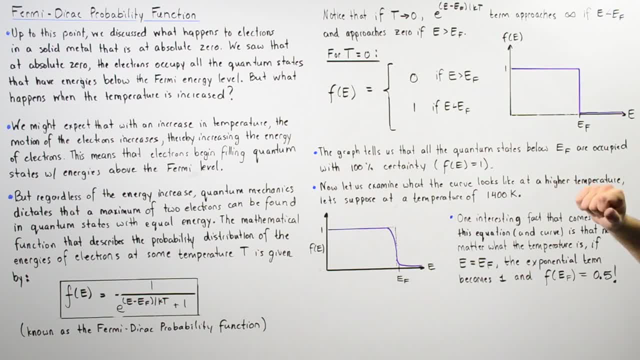 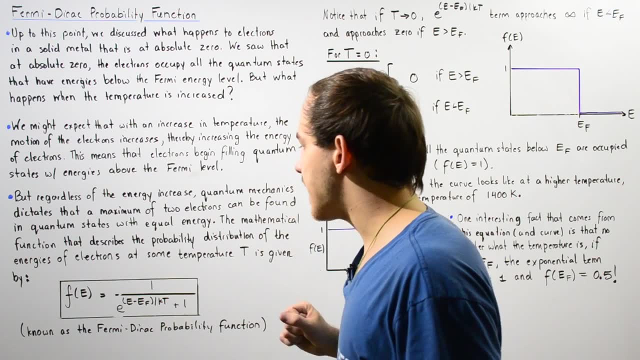 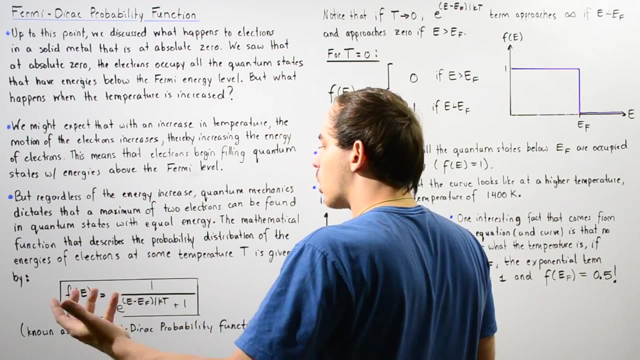 Now, on the other hand hand, if our t approaches zero and e is greater than the Fermi energy level, then if we follow the same exact procedure, we see that now this quantity becomes infinitely large, and one divided by a very large number is approximately equal to zero. So, in such a case, our probability 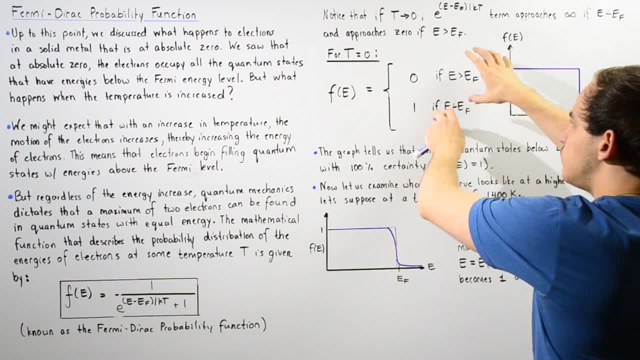 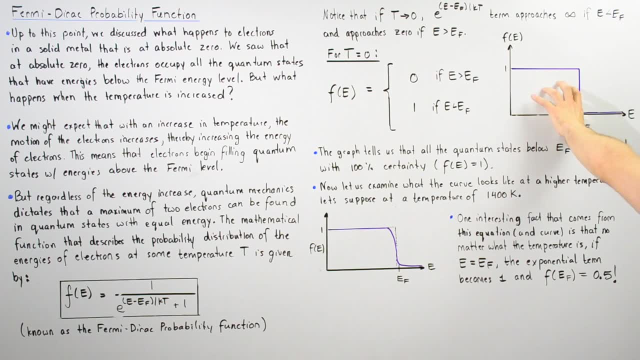 distribution is given by zero. So if we want to, we can actually plot this discontinuous function And that is given by the following quantity, the following graph. So, basically, we have our y-axis, which is our probability distribution f of e, and our x-axis gives us our energy. So we see. 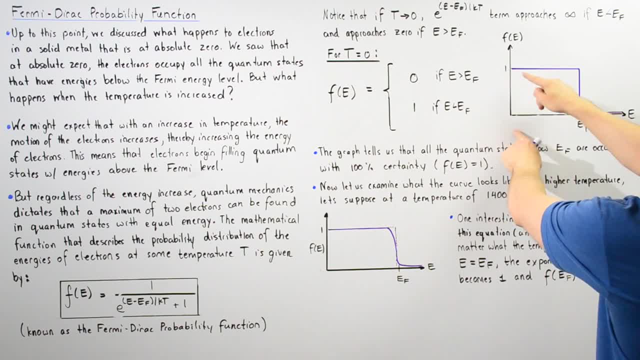 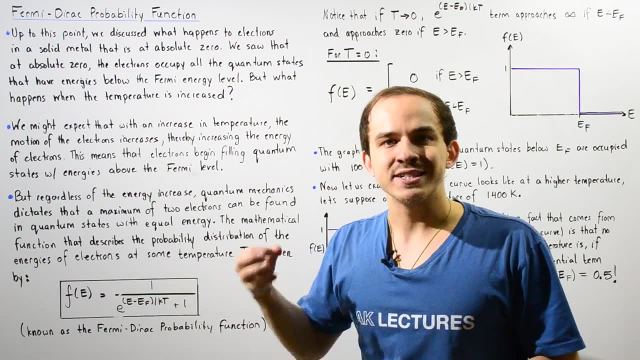 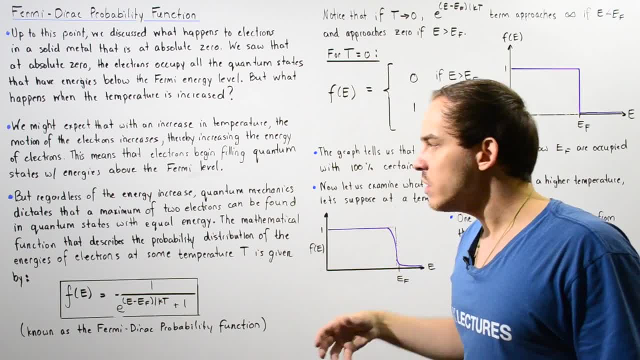 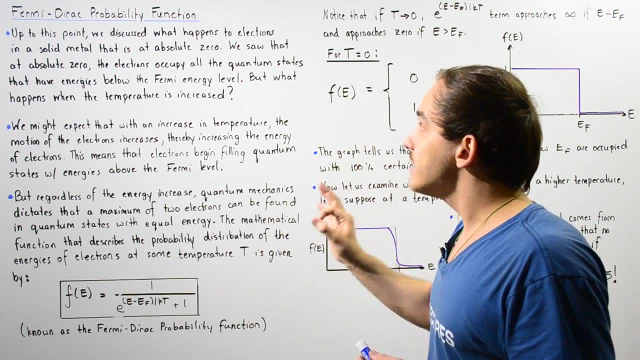 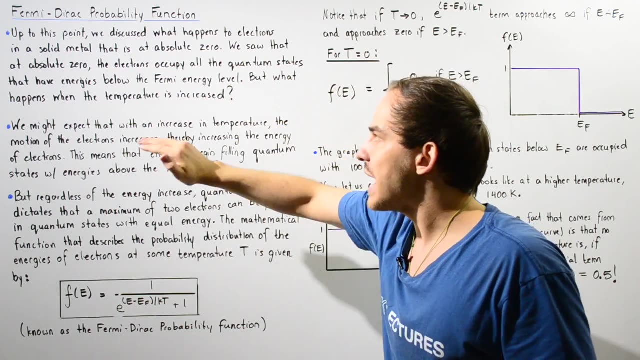 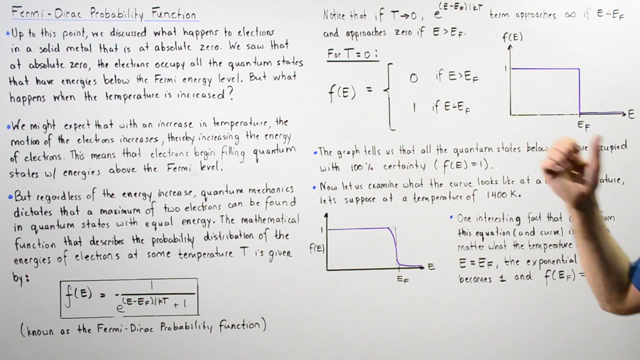 quantum states with these energies are completely filled. So this basically coincides with what we discussed in the previous lecture. we said that at a temperature of absolute zero the electrons occupy all the quantum states that have energies below the Fermi energy level, as described by the following graph. So the graph tells us that all quantum states below 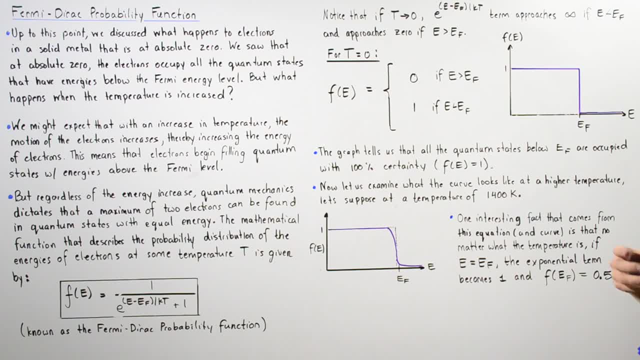 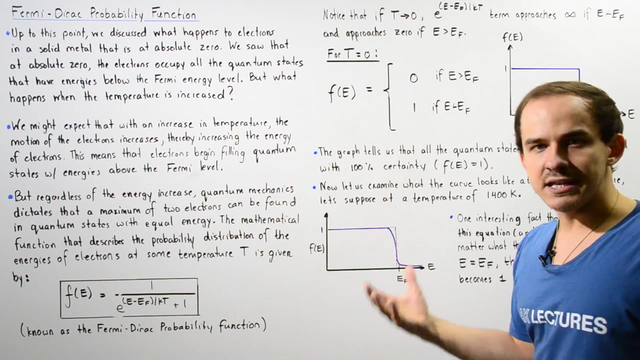 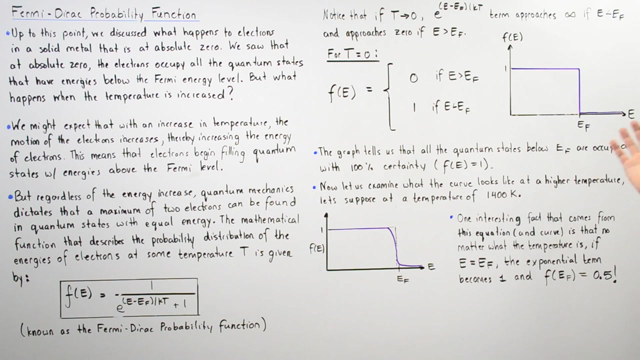 the Fermi energy level, EF, are completely occupied with 100% certainty, with a probability that is equal to one, And we see that anywhere above our Fermi energy level the probability drops to zero. So that means all the electrons are found in quantum states that are below this Fermi energy. 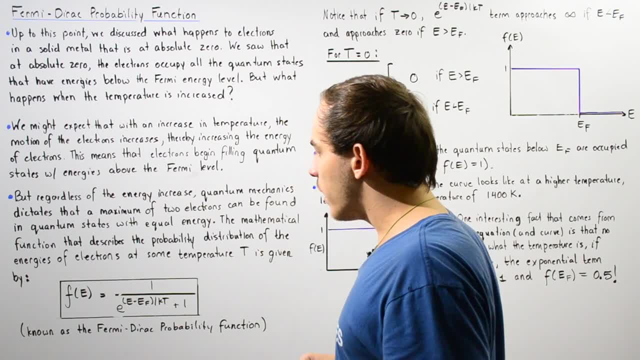 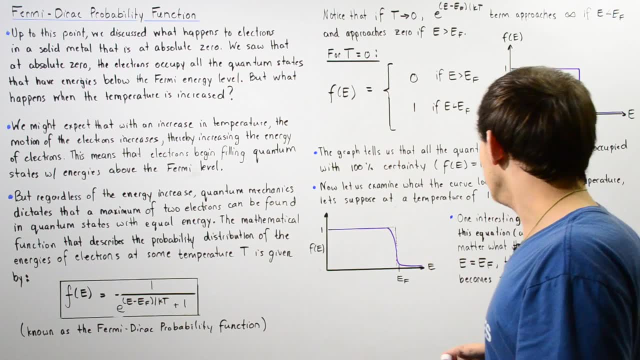 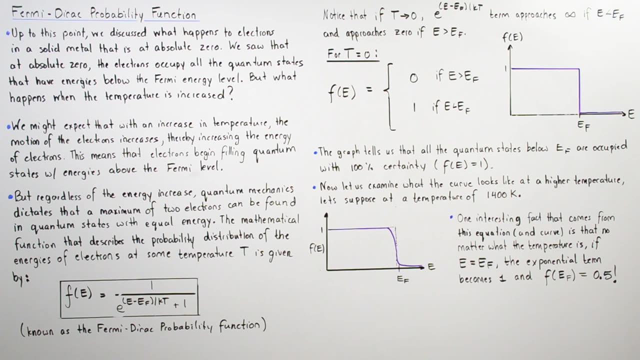 level. Now let's actually take this equation And let's see what happens if we increase our temperature from, let's say, zero Kelvin to, let's say, 1400 Kelvin. So now let us examine what the curve looks like at a higher temperature, let's suppose at a temperature of 1400 Kelvin. So 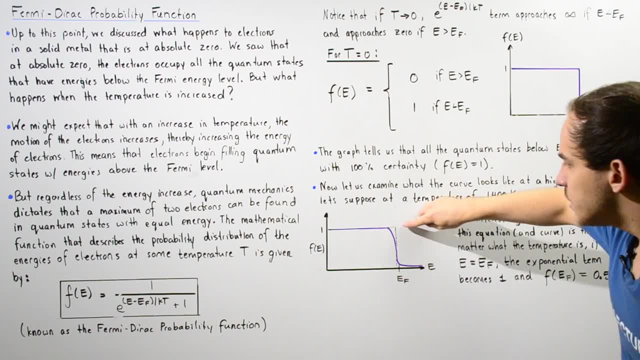 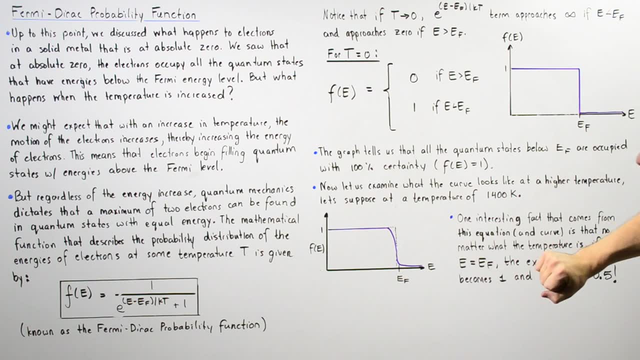 basically we get the following curve: So this dashed line shown in black. basically we get the following curve: So this dashed line shown in black basically represents this curve here. So we place that in there so that we can compare these two. 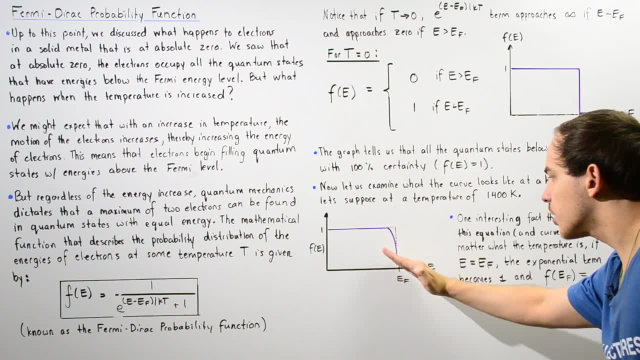 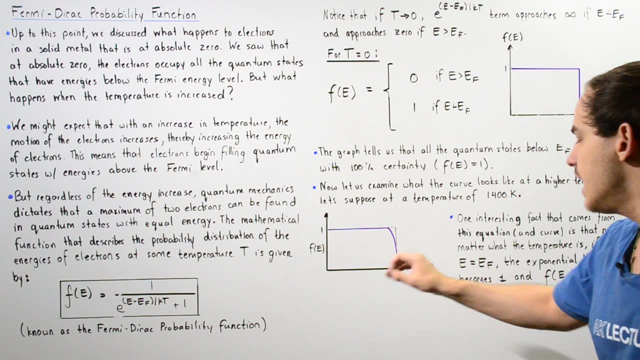 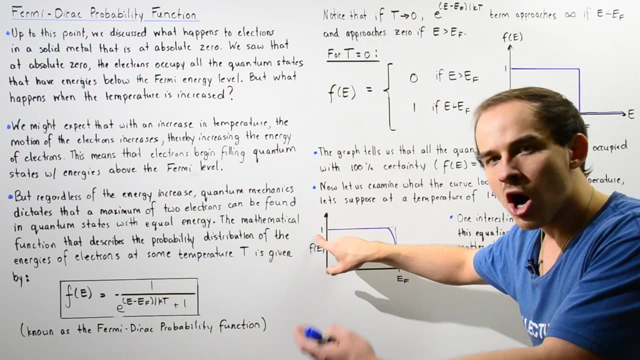 curves. So notice we have a slight curve, as shown by the following diagram. So the y axis is still our probability density f of e and the x axis is still our energy. So this is still equal to one where one represents 100% probability of finding our electron within that region. 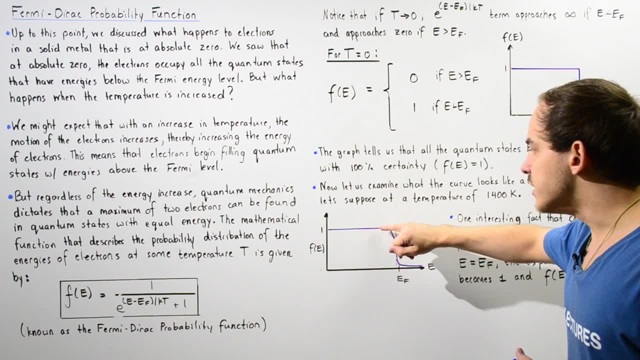 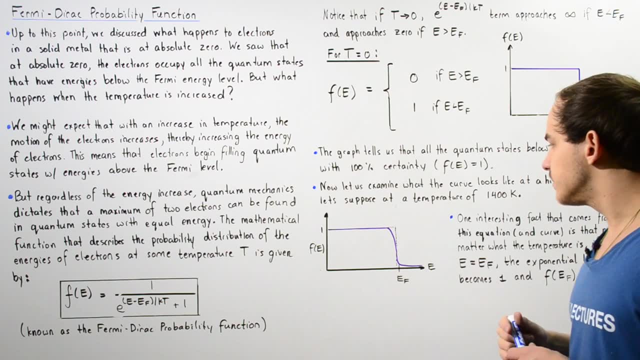 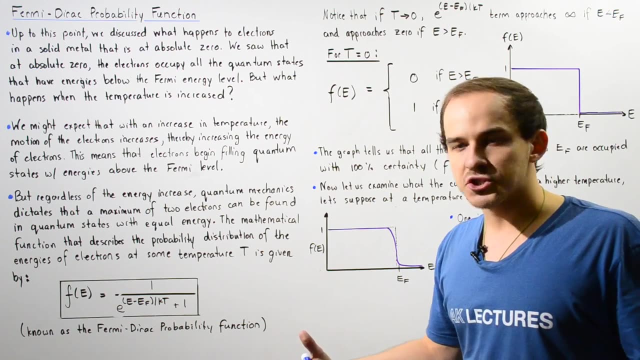 So basically we see, although within this region we still have 100% certainty of finding our electron within those quantum states, But if we examine this region here, we see that our probability actually drops. Now there's also one interesting thing that we see. So at an energy of 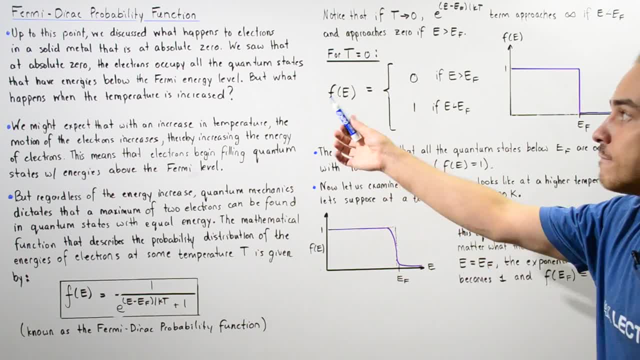 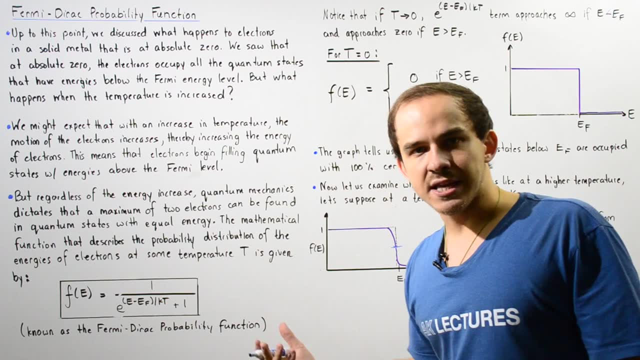 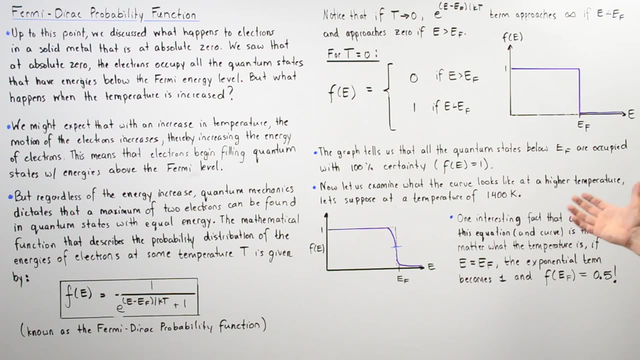 EF when our energy E is equal to the Fermi energy level. we see that our energy E is equal to the Fermi energy level. we see that our energy E is equal to the Fermi energy level. we see that our probability is exactly 50%. Our probability is exactly 0.5.. So, once again, one interesting fact. 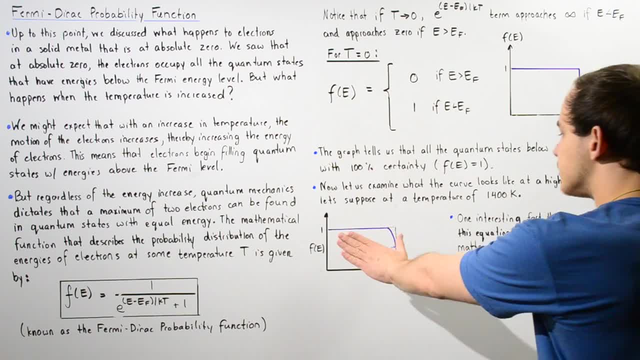 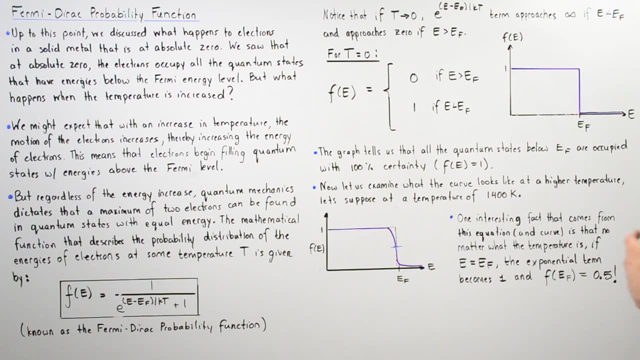 that comes from our equation as well as from this curve, is that, no matter what temperature we have, if it's 1400 Kelvin, 500 Kelvin, 10,000 Kelvin and so on, we see that if our energy of the electron is, 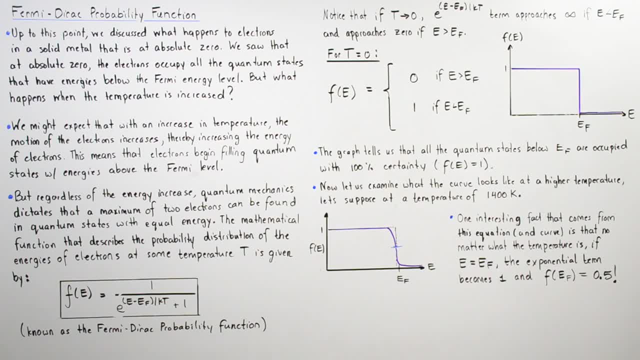 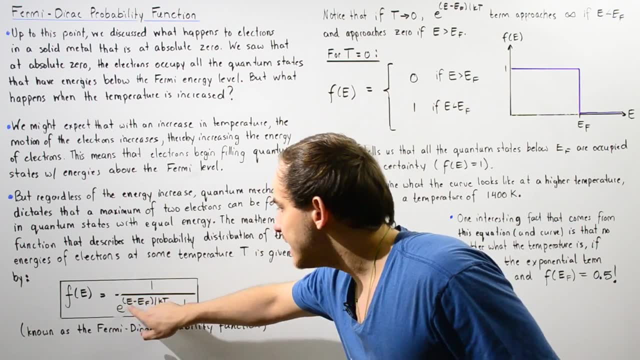 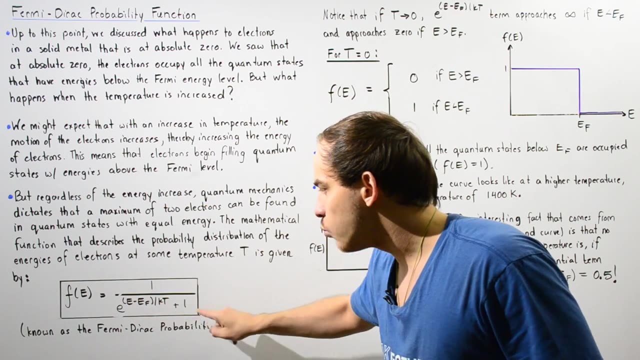 equal to the Fermi energy level, EF, then the exponential term in this equation becomes 1.. So if E is equal to EF, we have E to the power of 0, which is 1.. And 1 divided by 1 plus 1 is 1 divided.